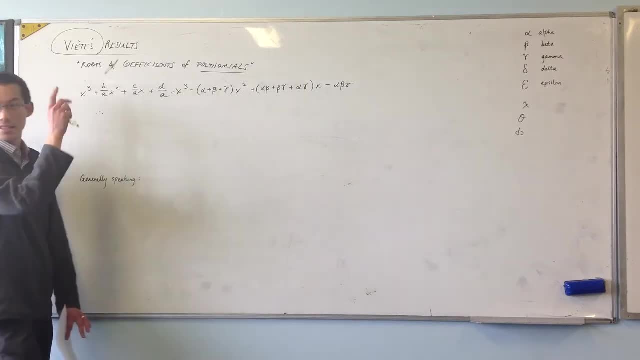 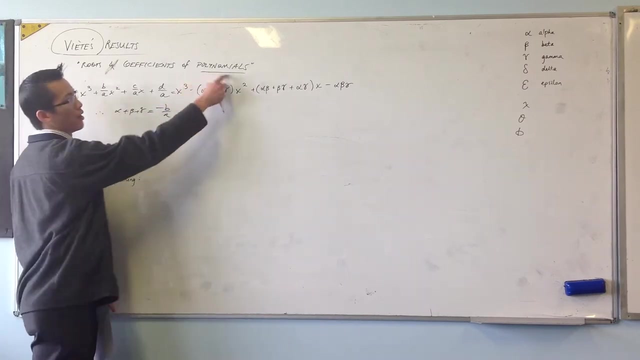 So, as you can see, what have I got here? First up there's the sum of roots, right, Alpha plus beta plus gamma, and, taking the negative over the other side, minus b on a. Now you're starting to see why sum and product of roots is not quite a good enough way to describe when you're going for polynomials, okay. 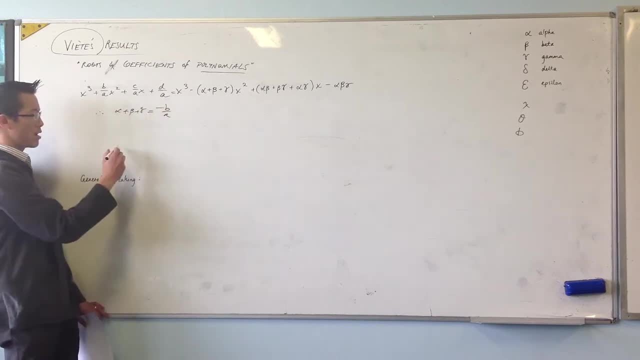 Because this is the sum of roots and looking on the end, there you've got the product of roots, which is minus d on a. But what's this guy? What do you call him? right, He's not the sum and he's not the product. 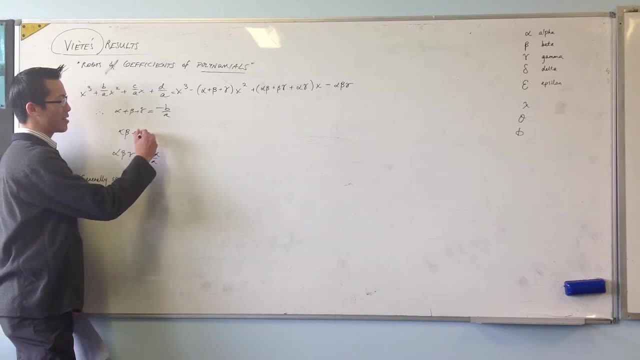 Yeah, so what we say, the way we describe this, which is c on a. If you want to say this generally speaking, okay, because you should be- it should look suspicious to you. You're like this is exactly the same thing that we got with the quadratic right. 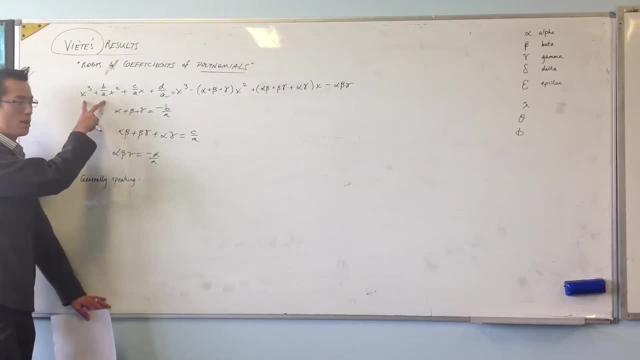 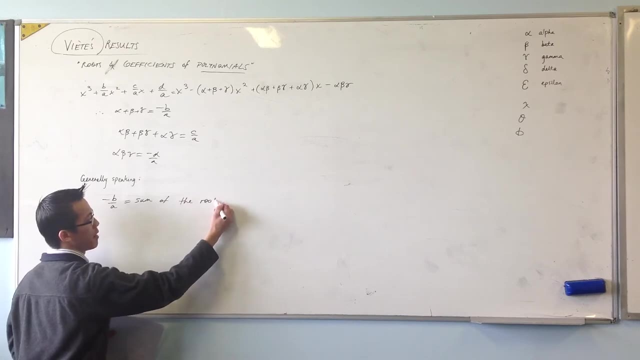 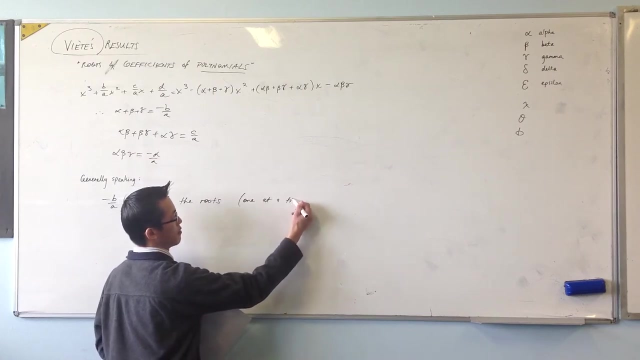 Minus b on a right, These first two coefficients. Here they're always going to be equal to the sum of the roots. but more specifically you say taking them one at a time, right? Hence alpha plus beta plus, gamma plus delta plus, however far you want to go right. 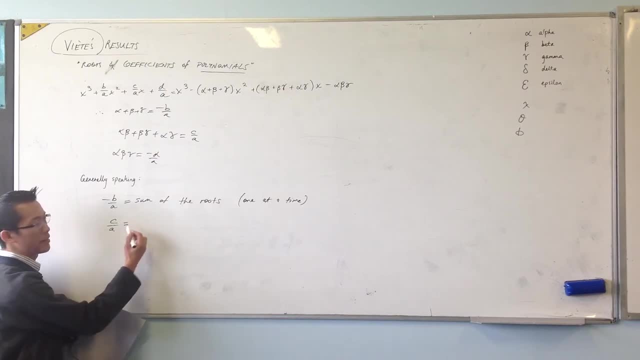 When you move up one c on a and please, please, please, watch out for the negatives. okay, Everyone always screws that up because it's easy to forget that it's there or it's not there. c on a is still the sum of the roots, sort of. 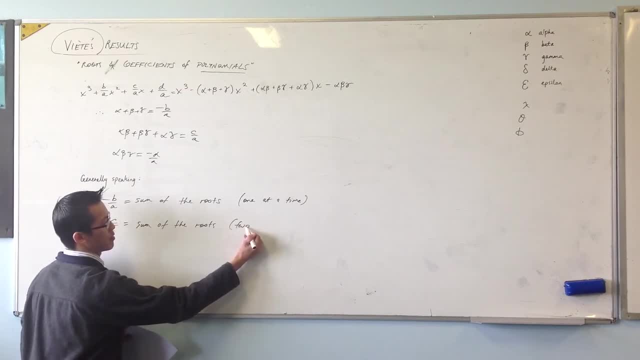 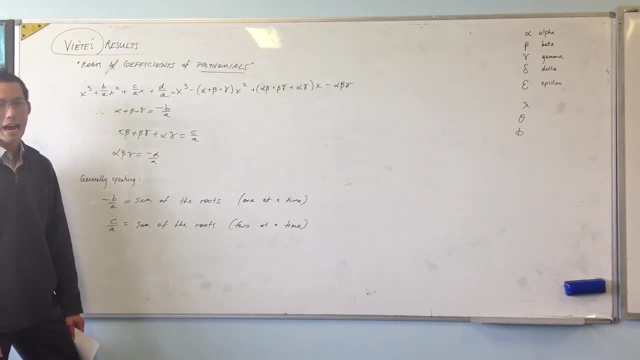 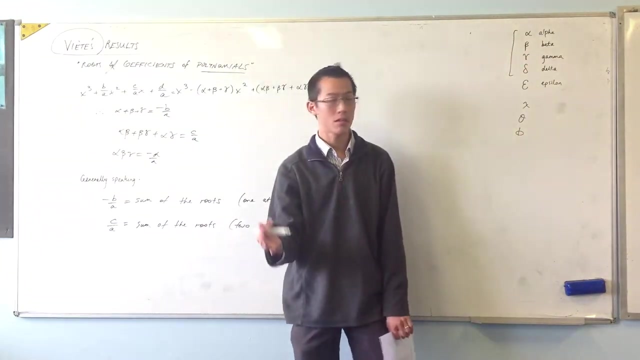 It's the sum of the roots, two at a time. Okay, So in this case it's alpha beta plus beta gamma plus alpha gamma. But for instance, if we had a quartic power of four, not power of three, right? 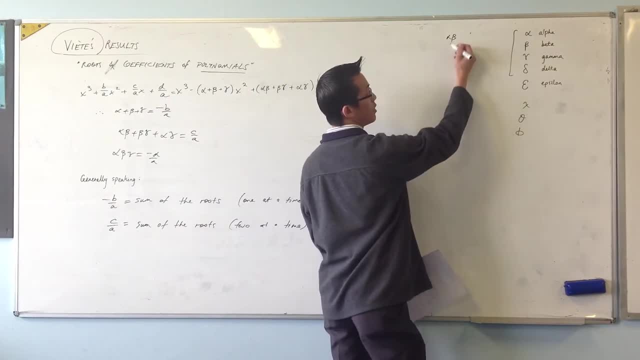 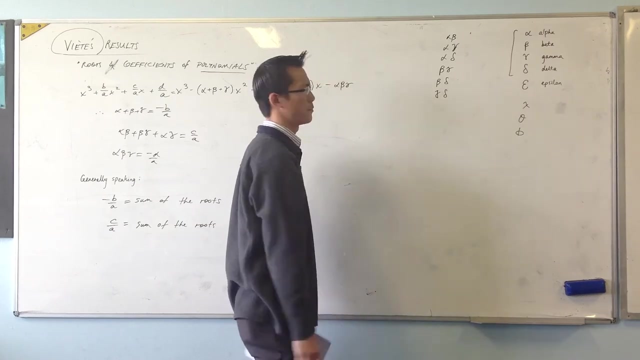 There would be many more combinations. right, You'd get alpha beta, alpha gamma, sorry, Bad gamma, Alpha delta. then you'd get beta, gamma, beta delta. you're going to get gamma delta. and wait, is that it? 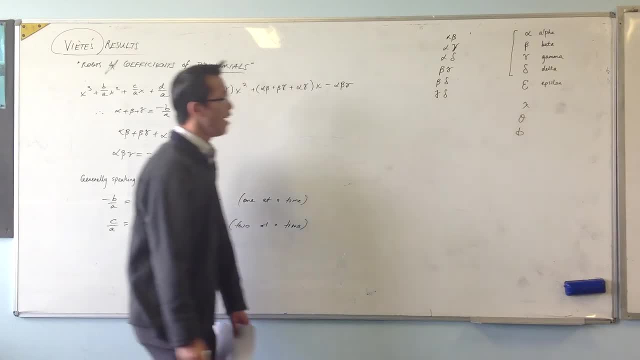 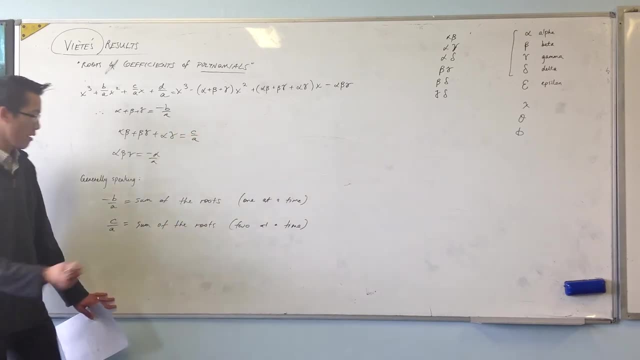 Yeah, Is that it? I think that's it right. Yeah, Now I've got them all, So you've just got to be careful and methodical in the way that you write them out so you catch every one. But that would be c on a if it was a quartic.